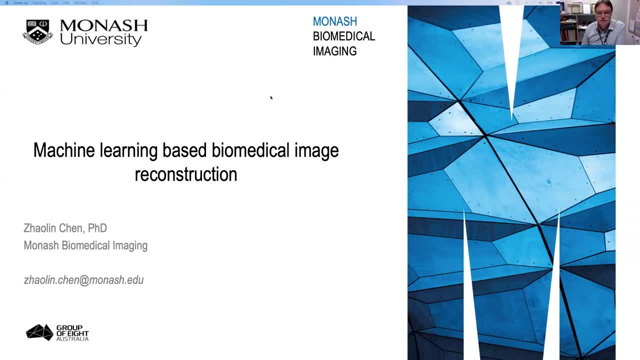 And these will be answered at the end of this very presentation. I'll just ask you all in those questions: The chat session, the chat section, is on the Q&A and has been disabled for everyone. So if you want to ask a question, you'll have. 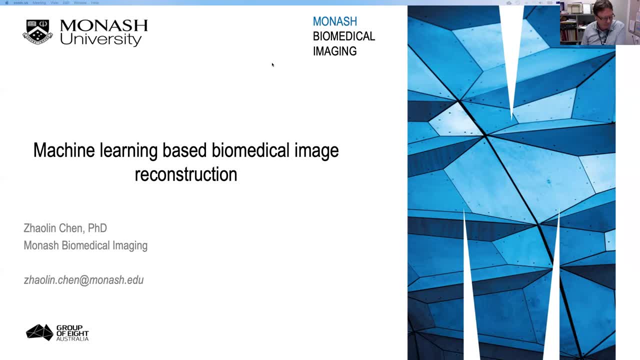 to type it in the Q&A and I'll monitor that as we go along. It's a genuine pleasure to introduce Dr Xiaolin Chen, who's our speaker today. Xiaolin received his PhD at Monash Uni in 2007.. He then had a postdoctoral stint at the Florey Institute. 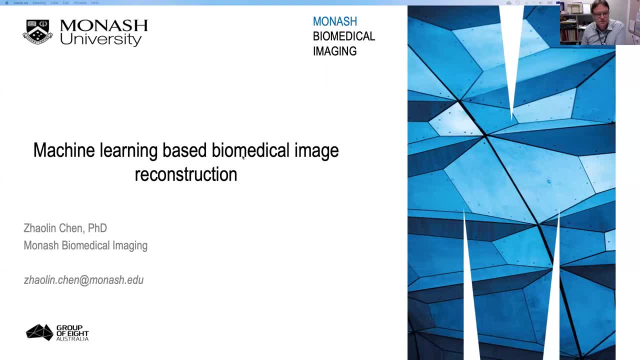 for Neuroscience and then went overseas to the United States to study at the University of the Netherlands, to a commercial entity of Philips Healthcare And there he instigated a lot of patents, did a lot of commercial work. He was recruited back in 2014 to his 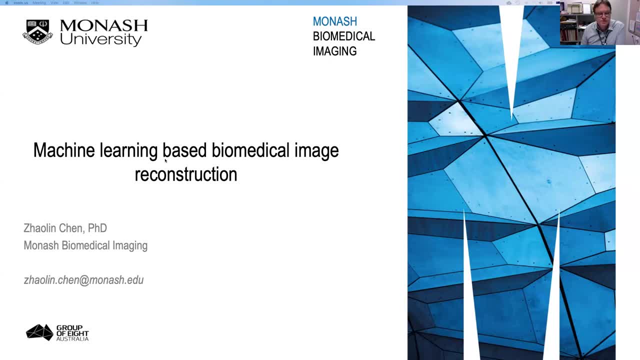 current position at Monash Biomedical Imaging, where he heads the image analysis team. He's authored over 60 peer-reviewed papers and has over 10 patents for his work, So he's an expert in commercializing. Dr Xiaolin Chen is an expert in commercializing and applying his research, And it's a genuine pleasure. 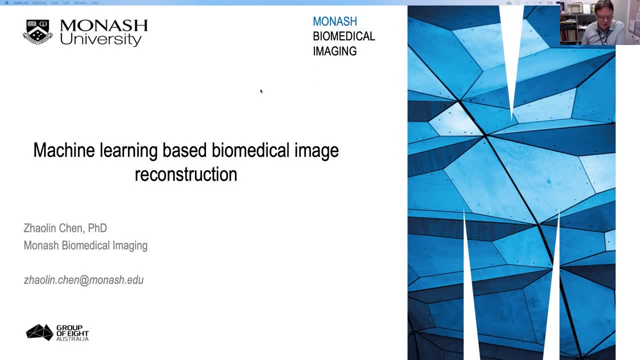 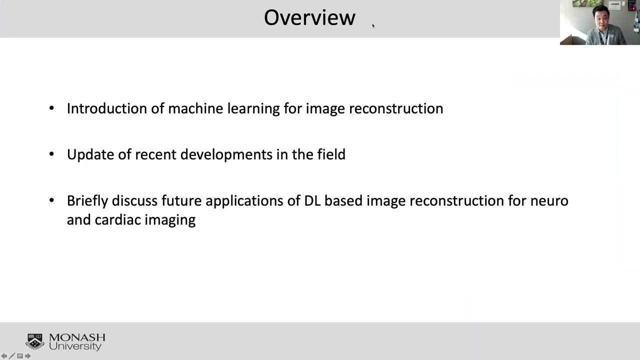 to welcome him today to present his talk on machine learning based biomedical image reconstruction. Welcome, Xiaolin Xiaolin Chen. Thank you, Mike, And hello everyone. Welcome to our MBI seminar on machine learning based biomedical image reconstruction. So the overview of today's talk is about the 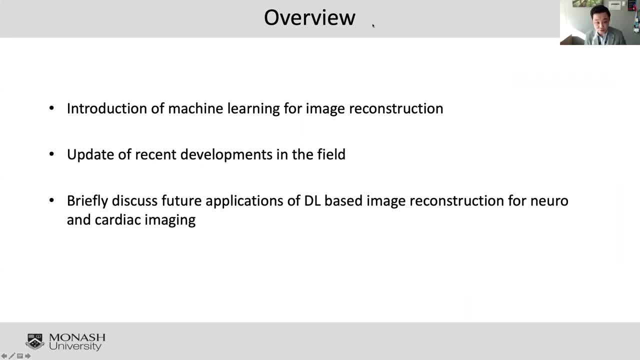 concept of machine learning. Okay, so I'll first introduce machine learning or image reconstruction. What is the problem? What is the relevance or machine learning for you, Recon crimson- And then I will update on the recent developments in the field And at the last I will briefly discuss future. 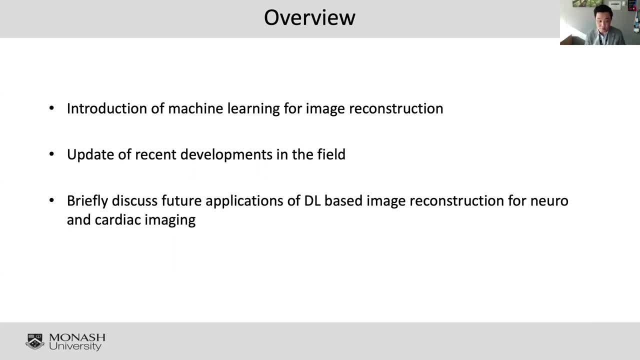 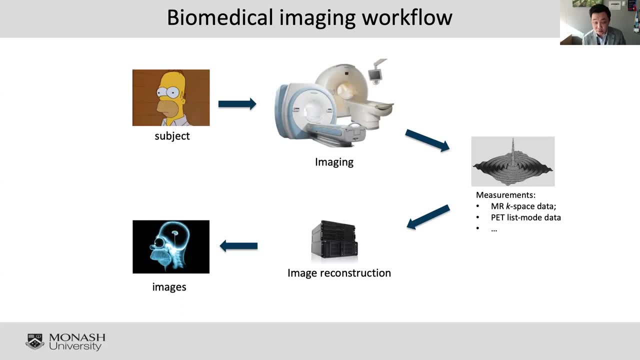 applications of bill based imagery construction for both neural and cardiac imaging applications. So here's the overview of a biomedical imaging workflow of a vaccine. Here we would like to pouvez explain a bit about the issue. that 궁금不到, Because it's difficult, There's immediately. 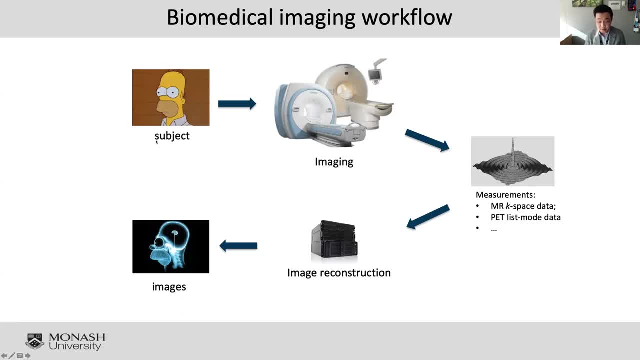 already in contact. I am your next speaker. Please To walk me over to our talk talk. we have a subject- participants or patients- and we got an imaging system. so the subject is inside the imaging system and then the the measurements is acquired through the experiments. so, in terms of measurements, we have MRI case-based data. 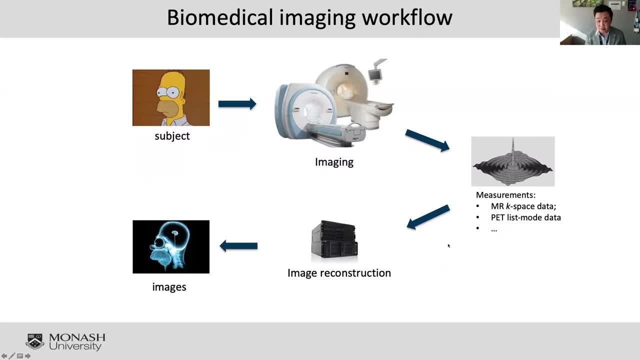 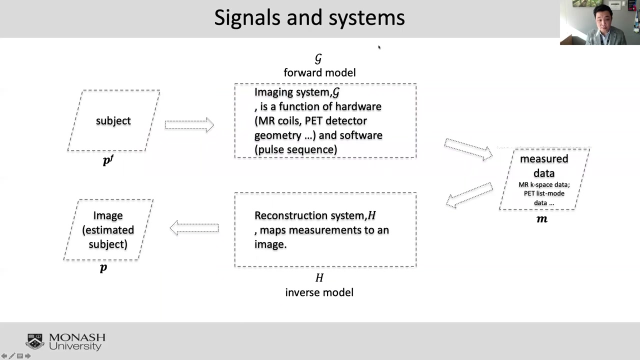 or PET, this small data, and then the raw measurements will go through image reconstruction and then we generate the image of the subject. so this is a overview of the complete workflow in terms of imaging and the reconstruction. so if you look at closely, what are the signals and the systems, how we can model. 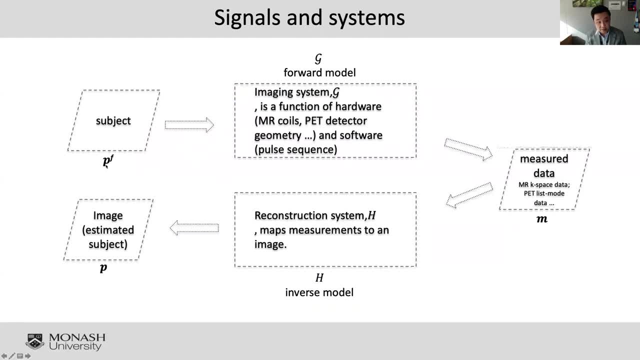 each of these elements. so we have a subject- let's call it PF- which is the ground truth, and we have a forward model which is G, and we have a forward model which is G, and we have a forward model which is G, which represents the imaging system, and G is a function of hardware and 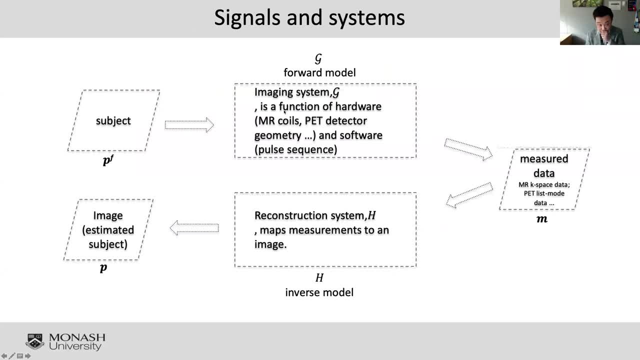 software. so the hardware includes MRI coils, PET detector and software in terms of MRI will be part sequences and then, through the imaging system modeled by G, we have a measurements. let's call M again, that's case-based small data, and then the key part for today's talk will be around reconstruction system. 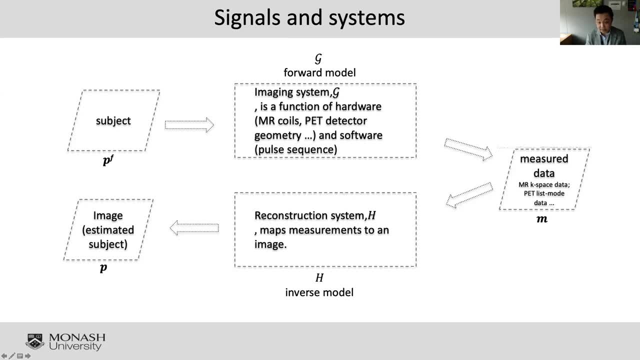 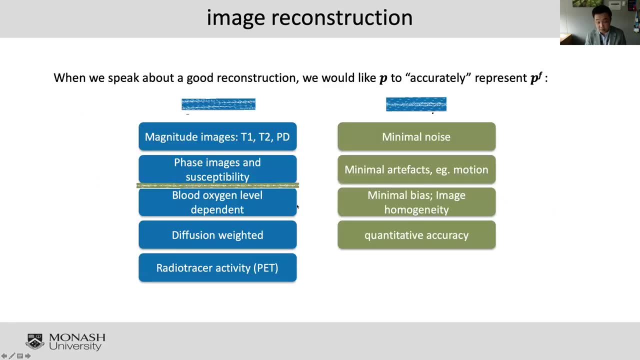 how we can design a optimal reconstruction system that maps measurement to an image. so back to P, in terms of the, when we speak about a good reconstruction, we would like P to accurately represent PF. so in terms of the, the reconstruction, the P, it can be magnitude images, for example, T1-weighted, T2-weighted. 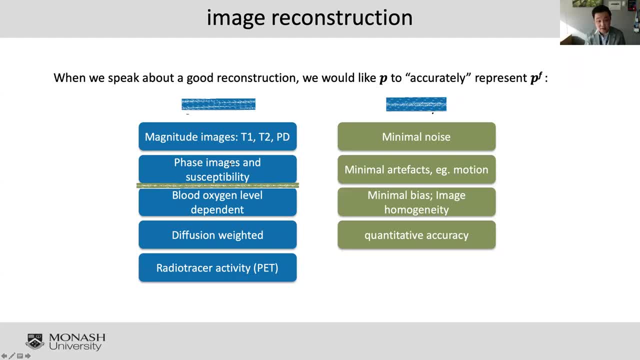 polar density-weighted or face images sensibility-weighted or both. signal diffusion-weighted or in terms of PET, would be trace activity distribution. So the accuracy I mentioned before. we would like P2 to accurately represent PF. The accuracy, normally the first thing we want. 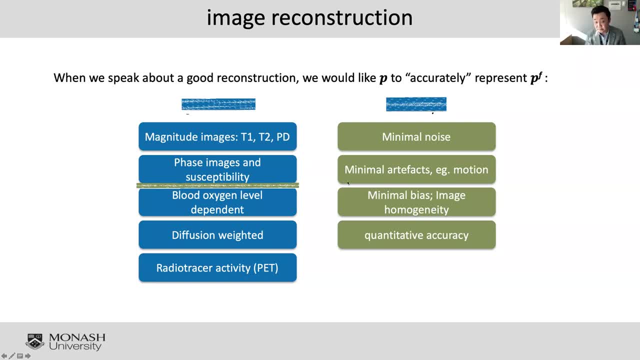 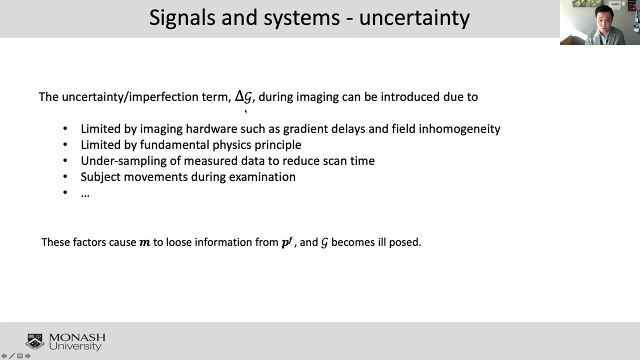 is minimal noise and minimal artifacts, for example motion and image homogeneity. So we want to have a good, uniform image and the quantitative accuracy. So you may wonder why we need to use machine learning. Can we just model G and calculate the inverse of that? 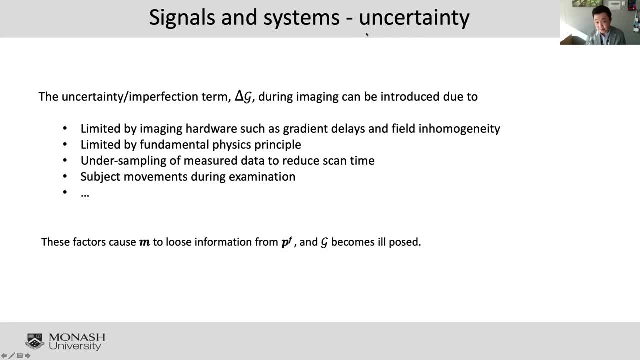 It actually comes from a term called uncertainty. So the uncertainty comes from multiple factors. So the uncertainty in the world is called imperfection. Let's call it RG. It can be introduced due to the limited imaging hardware, for example gradient delays, if you need homogeneity. 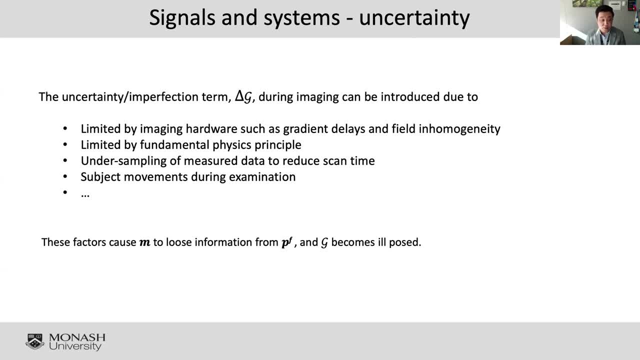 which is something the engineering limitation and also limited fundamental physics principles And also another popular limitation could be. we want to make the scan faster. we end the sample of the data And then subject movements during examination often occur, So all these factors will cause M to lose the information. 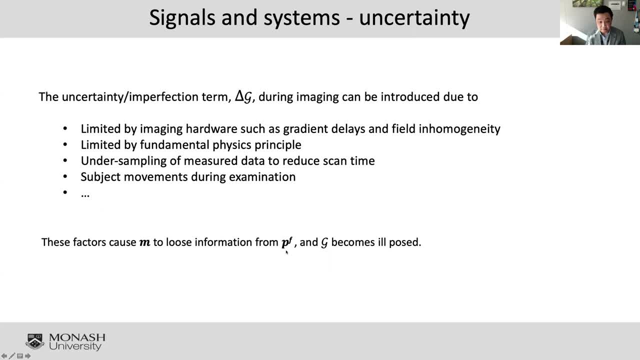 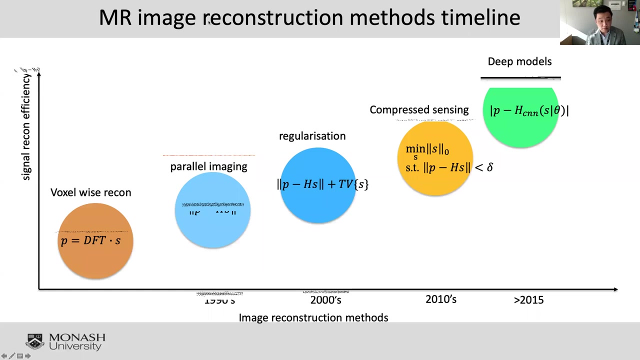 some sort from the ground truth, PF And consequently G becomes ill-posed problem. So the inverse of ill-posed problem is much more difficult. That's where machine learning, and especially deep learning, can help a lot in this context. So if we look at the MRI image reconduction methods, development over the years, 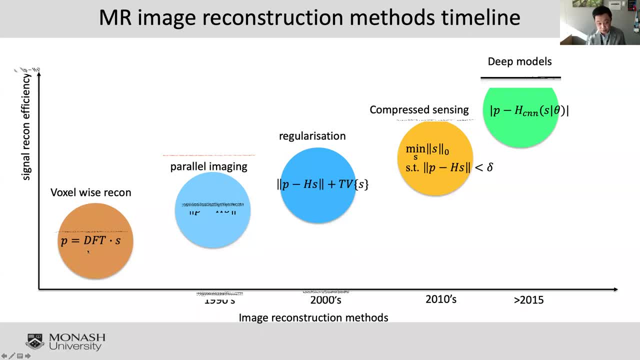 So initially we have a Fourier transform reconduction, early days of MRI. The Fourier transform is applied to the measurements and then we reconduct an image And during 1990s the parallel imaging technique becomes popular. So the parallel imaging techniques. 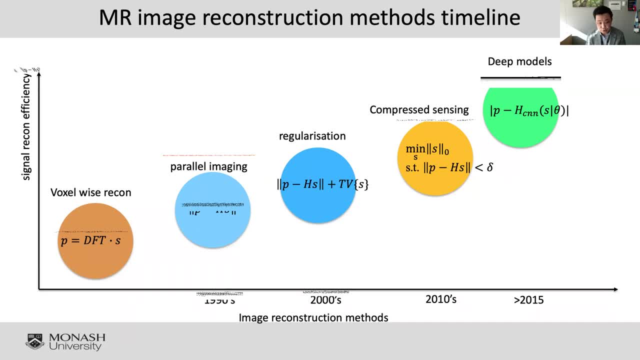 is addressing the under sampling issue. And then we calculate the inverse in a optimization problem: P minus HS. so P is your measurement, that is the ground truth, And H is your inverse system, S your measurements again, And then you can calculate in a more optimization way. 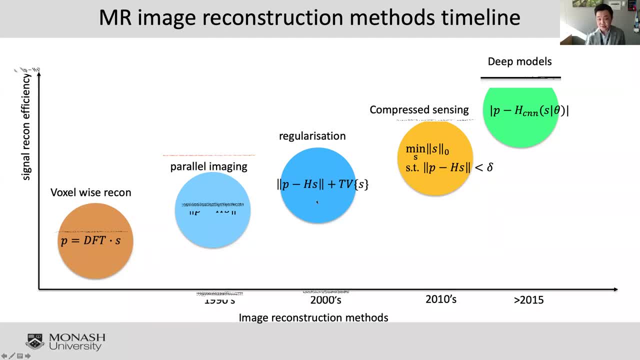 And then in early 2000, the regularization becomes popular. So on top of parallel imaging we apply a regularized term here If we know any prior information on the measurements. one popular technique is to use total variation to regularize, to reduce noise substantially from the recontracted. 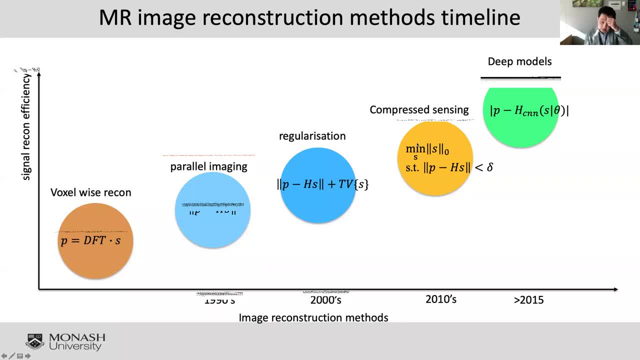 image And then, around 2010 and onwards, complex sensing becomes an important topic to accelerate MRI. So complex sensing is a technique that uses sparsity assumptions with the image and then recontracting the image, assuming the image is sparsely represented, and then we can. 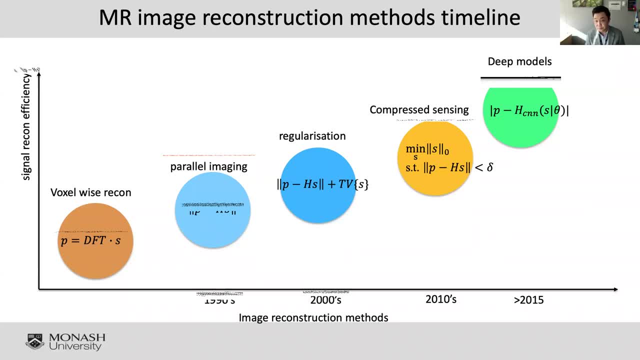 leverage that as a strong prior to recontracting the image. In 2015 and onwards, deep models will start becoming a useful technique for recontracting images. So, unprincipled, All the previous techniques are shallow networks, are shallow models. 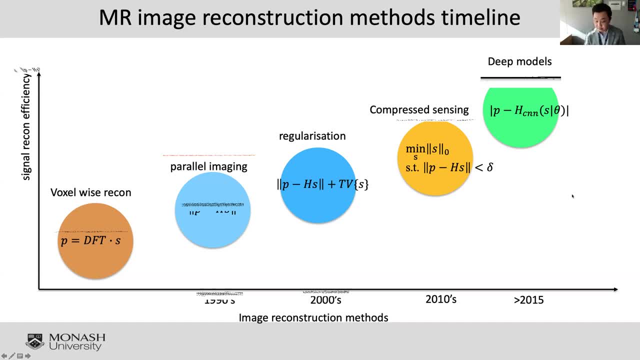 The edge are simple: it can be linear, non-linear, but only if it's a few parameters. But once it comes to deeper models- edge neural networks, that contains millions of parameters, Parameterization, optimization, becoming a lot of them. So that's the development. 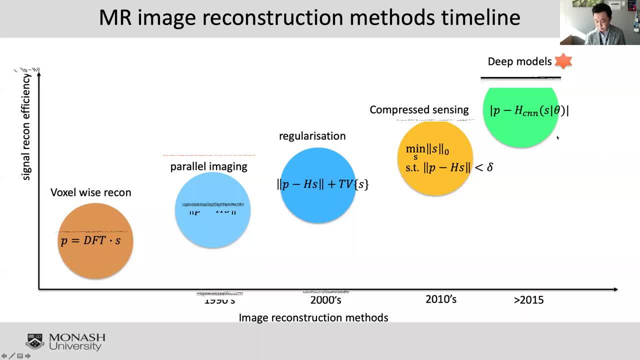 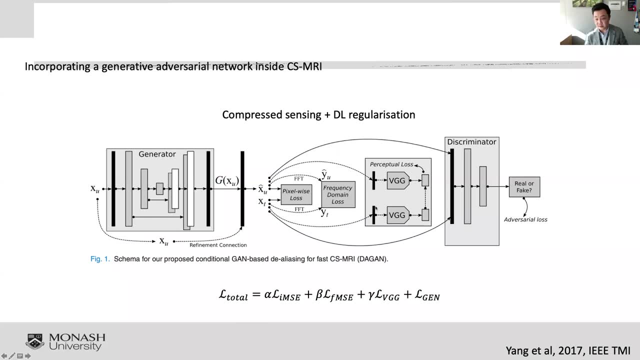 and this talk will be mainly around deep models or look at deep learning, recent development in this field and up to around that topic and some of our development in this field as well. So this is the regularized deep learning, So the initial attempt, Young et al in 2017,. 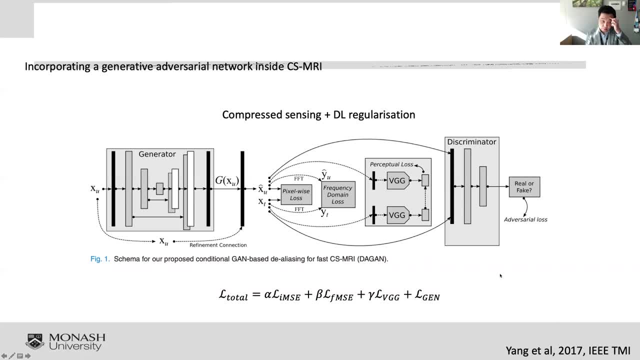 developed a technique and published in HLB-PMI. So they incorporate the deep learning network within the deep learning network. So they incorporate the deep learning network within the deep learning network. So they incorporate the deep learning network within the Compressensing reconstruction. 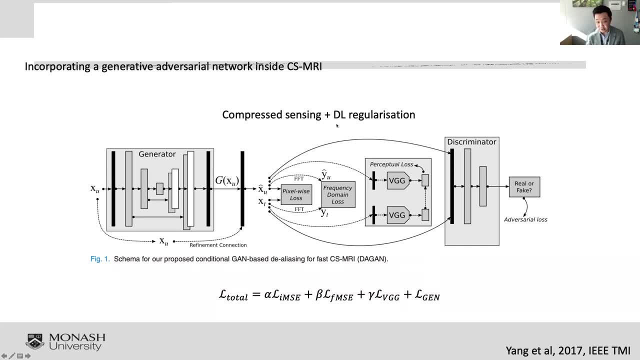 So it becomes a Compressensing plus a DL regularization, And the particular network that they use was a generative-adversary network, So it's called GAN and then that's embedded into CS MRI- Compressensing MRI- to further improve the image quality. 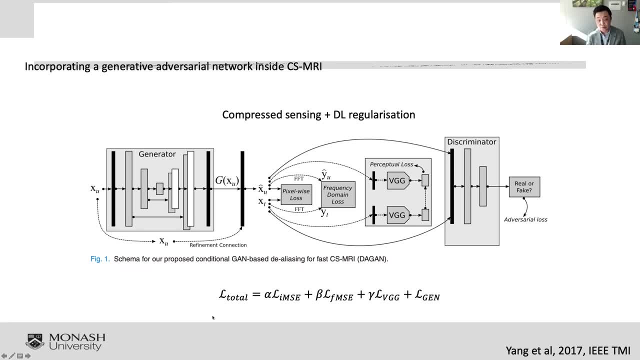 and the speed of the data. So they have designed a special loss function for their network. So a total loss function equals image space. loss function mean square error, pixel-wise loss function, as shown here, and then a frequency loss function as well. 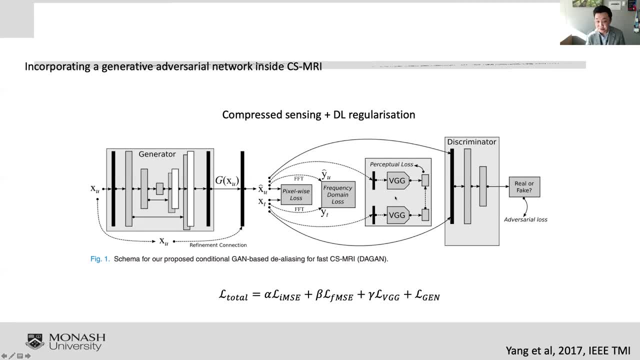 And also a perceptual loss to look at the image, similarity between the recontracted and the ground truth image and, of course, a generative loss. So that's the early attempt to combine deep learning inside a Compressensing reconstruction. So in 2018, Zhu et al. 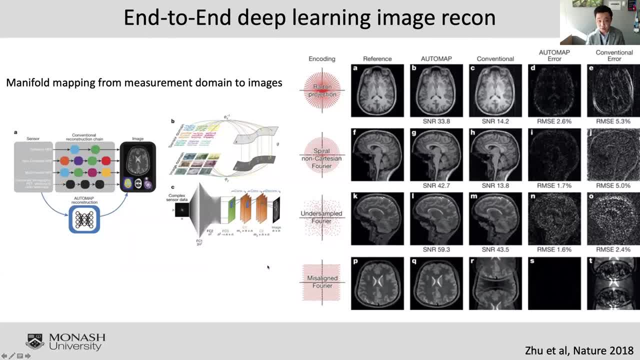 made a more ambitious approach to use deep learning for image reconstruction. So they basically map the measurements completely from the measurement space to image, end to end. Okay, so during that process, the case space, for example, if it's MRI- mapped directly to the image. 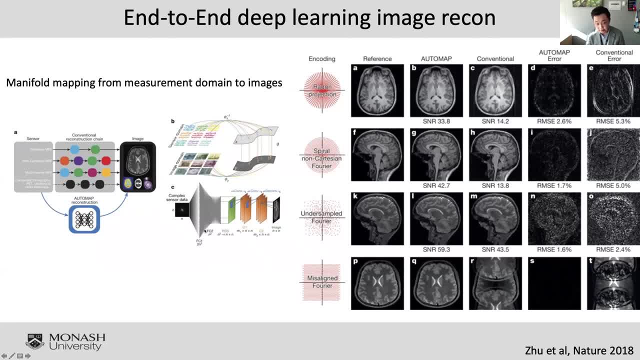 then they introduce a fully connected layer to model the Fourier transform and then map the complex sensor data, which is case space, into the image. So this is the work and the model they use and they have tested in different case space trajectories. 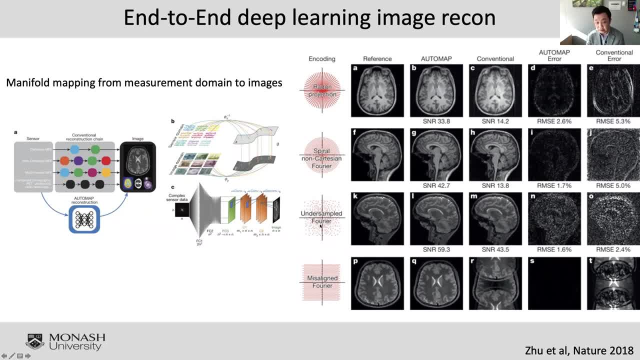 for example radio spiral, and also heavily under-sampled case space data, or with some artifacts as well. For example, here is this gradient, imperfection, delays and so on. So they compare their technique. it's called the AutoMAT in this row, as you can see. 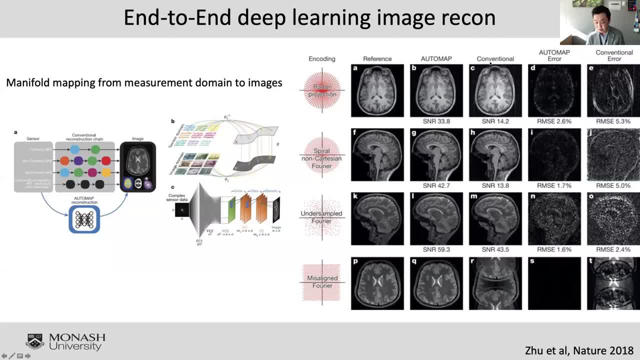 and then with the conventional techniques state of the art prior deep learning. So they have demonstrated that AutoMAT recontracts better in terms of mean square error compared with conventional technique. So in different trajectories, also in heavily under-sampled data. 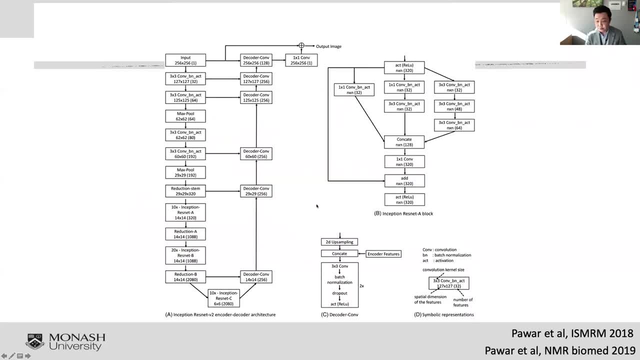 Yeah, okay, So we also take an adventure in this. in around 2017, Camlash developed this end-to-end approach for motion corrected deep learning recontraction for MRI. So with the input- I'm not going into details If you're interested. 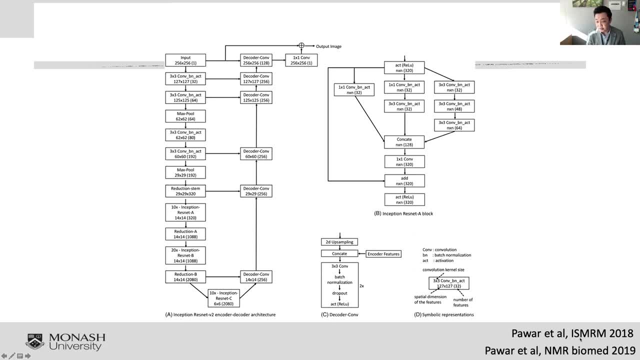 have a look at Camlash's paper published in both ASMR and AMR in Belmont. So basically it's a 2D network: We have an input and we have an output. The network architecture is a ResNet encoder-decoder architecture. 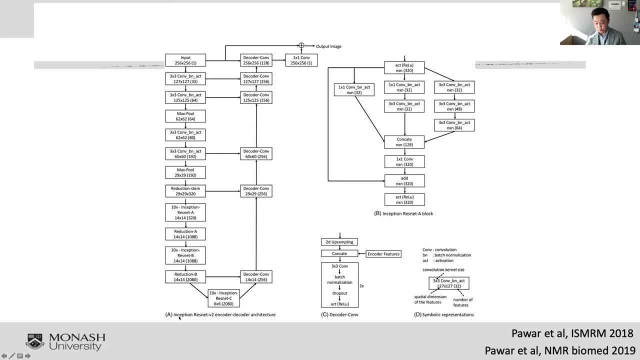 So with inception network we look at the multi-resolution aspects because motion can be a global artifact or a local artifact, depending on the perception, depending on the severity of the motion artifacts. So this network really captures the severity and the spread in the motion really well. 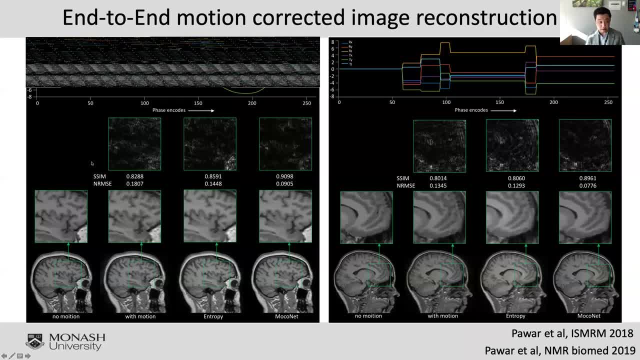 So we use this and demonstrates the improved motion correction. As you can see here we tested two scenarios. So the first scenario is with the slowly moving head movements And then we also look at abrupt motion, so sudden changes in the head position for neural examination. 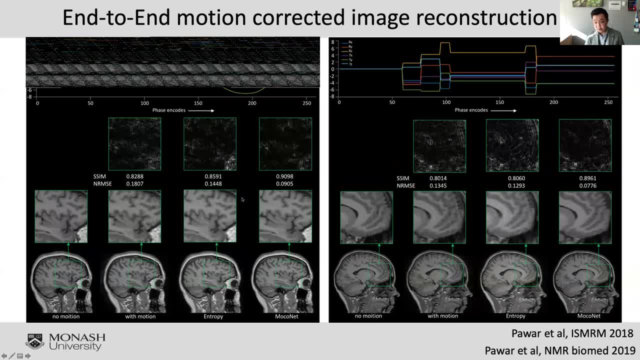 So we look at a slowly moving motion, in both scenarios The motion artifacts. if you compare the ground truth, which is the first one, and then with motion, you see this gives ring artifacts in the slow motion and a more sudden change of the image. 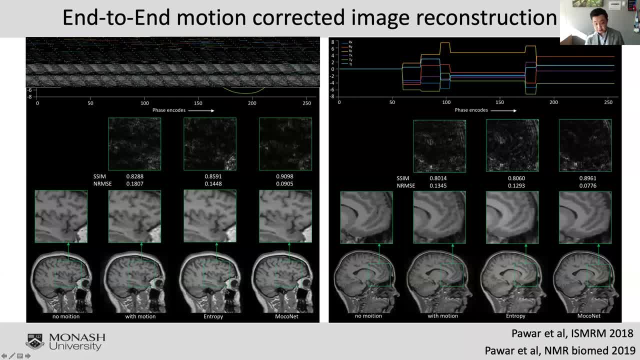 in the sudden motion And then we compare it with image-based technique for to correct motion, called entropy-based technique, And our technique we call MocoNag. MocoNag really improves the reduce the motion artifacts, suppressing the motion artifacts effectively. 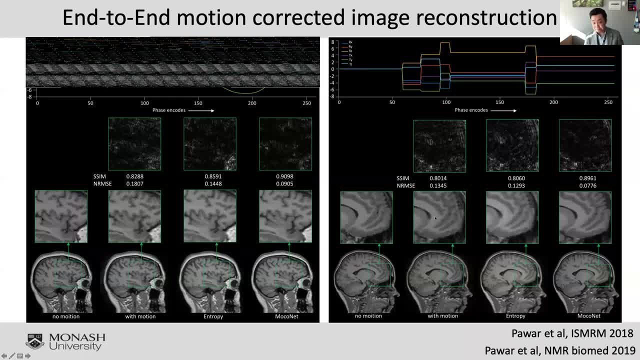 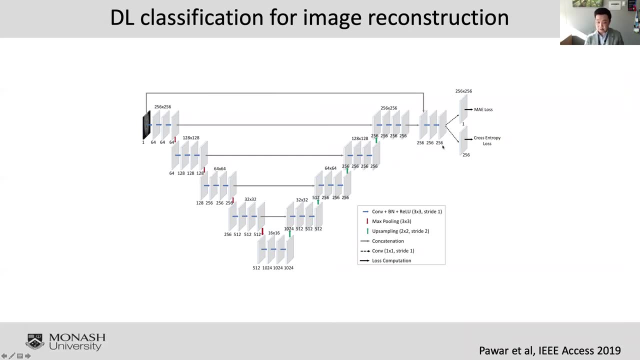 compared with the ground truth and the motion corrupted the image. So, and then we also further extend the network, we include different loss function to evaluate the image reconduction accuracy. So most of the people in the literature use a sort of regression loss function. 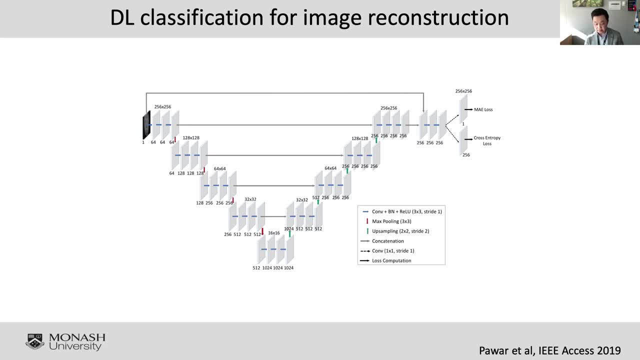 where we look at the neighborhood effects. We look at the loss function by summing up all the voxels in the image. The problem with that is you don't differentiate between image sharpness and the effectiveness of reducing noise. right A sharper image. 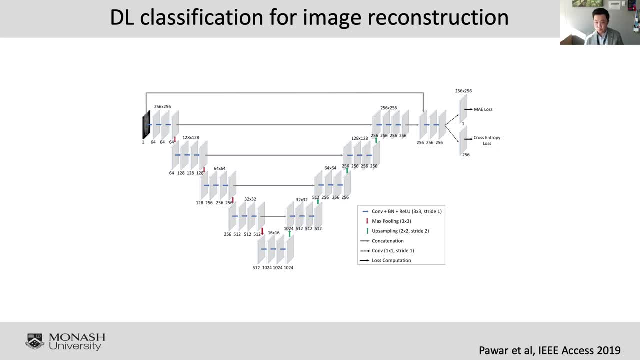 and a blurred image may give you a equal loss function in terms of regression, type of approach, When you look at the cross entropy, where the technique Kamlesh introduced later on, we look at per pixel. So we're basically using a classification, a classification network for image reconduction. 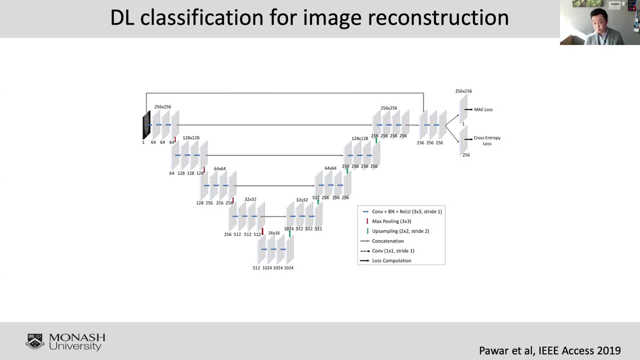 So the challenge here is the classification network per pixel will requires a lot of memory. So we have done a lot of parallelization and the way of look at images in block and also parallelize in terms of the depth, in terms of the, for example, MRI. 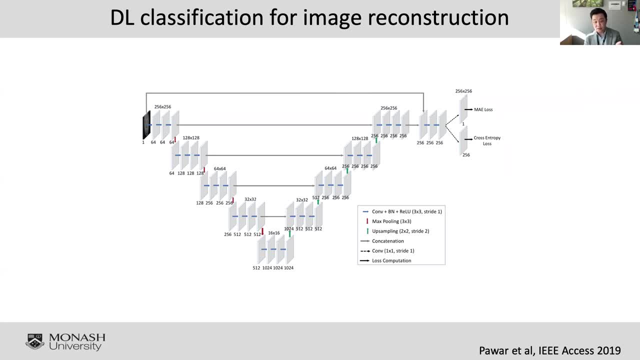 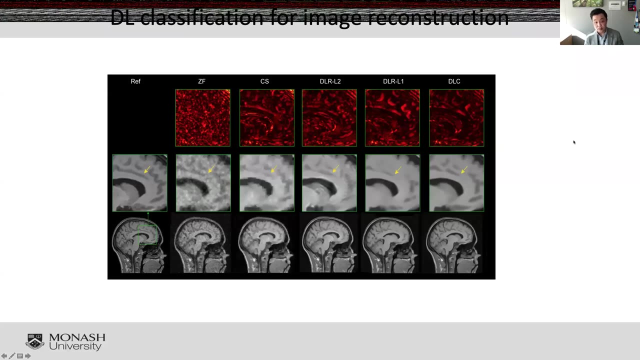 we normally have 16 bits of storage and then we can look at the per eight, eight bits as a segment and then that can be parallelized to speed up the reconduction And the image quality by using that approach is substantially improved compared with conventional. 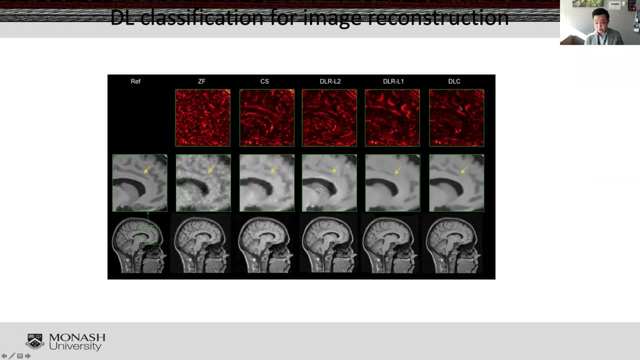 deep learning networks, regression-based deep learning networks. As you can see from here, the ILC is classification network. Kamlesh introduced, we used and in this case has seen brain imaging and compared with the reference and the zero-feeling reconduction which is 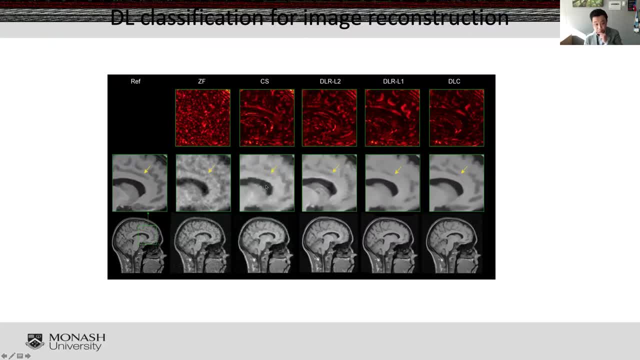 is the very early on technique and the compressed sensing which shows a blocky effects, artifacts and deep learning network. depending on different loss function, whether it's L2 or L1, they both regression-based loss and compare those with the classification loss. 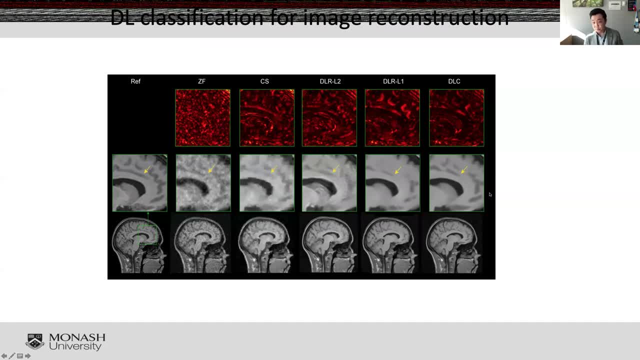 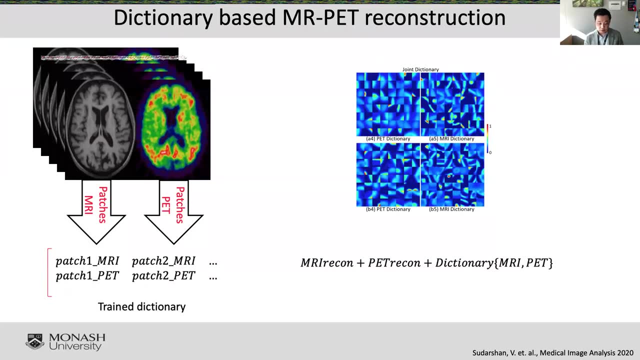 we see a better image quality overall and in both reducing noise and image sharpness. So I will move on to slightly different topic, but also using machine learning for imagery contraction. In this particular case, we look at MRR-PET imagery contraction. 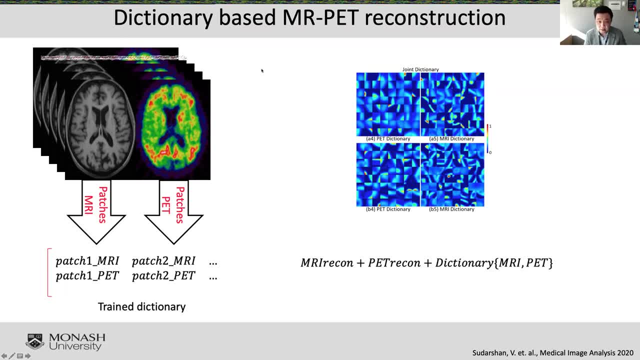 So MRR-PET is a scanner we installed at Monash Biomedical Imaging in 2016, and the stress of this scanner is acquired dual modality simultaneously. So we have an MRI and then we have a PET. So the 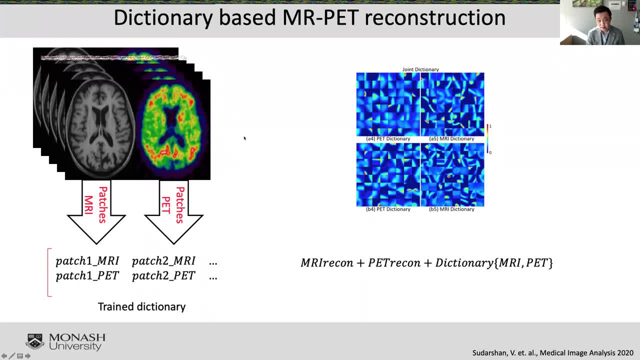 although the data is acquired simultaneously, the imagery contraction then separately inside the scanner. So we think we can do better in terms of merging and fusion the two modalities together. So this is a technique developed by Viswana, So he developed a dictionary-based. 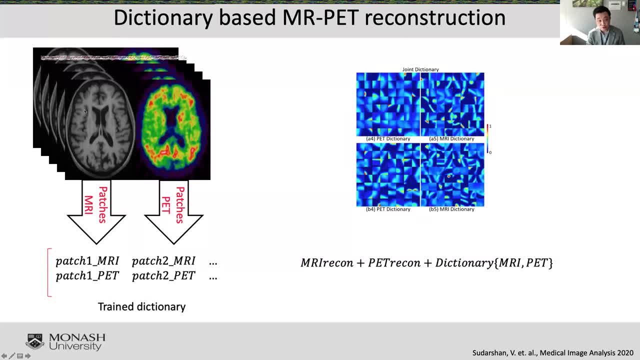 MRR-PET recontraction technique where we can extract patches, the corresponding MRR-PET into a dictionary form. So, as you can see, we put into a metrics where we have a different patch locations, so sort of a tensor setup. 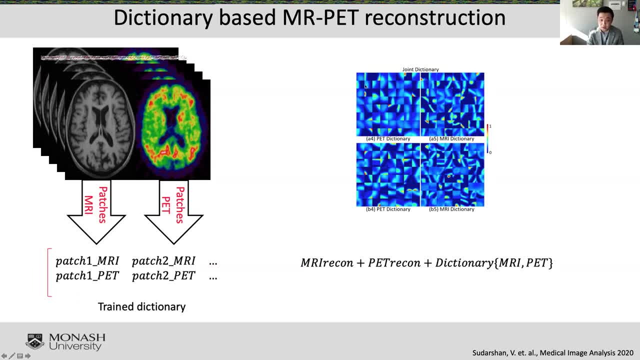 and then we can calculate a basis function and base non-negativity constraint. so all the priors are positive. So, and we can see here it's a little bit, it's like, let's just say it's a kind of normal image. 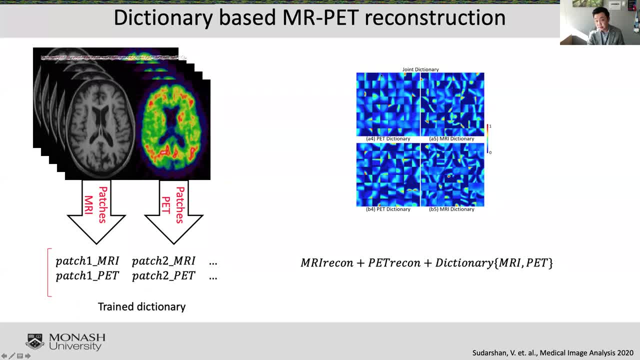 let's just say it's a kind of normal image And we can see MRI basis and the corresponding PET basis And the reconduction takes the following form: We have an MRI reconduction plus a PET reconduction, simultaneously regularized for both, based on dictionary. 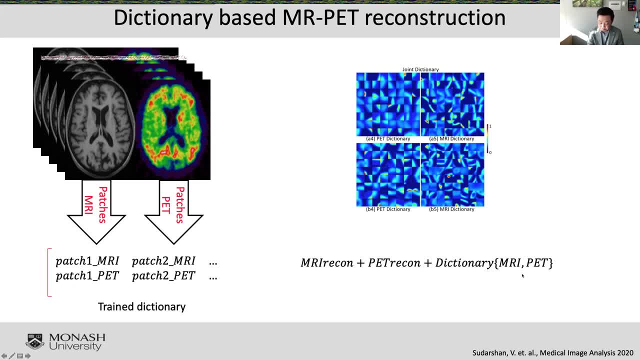 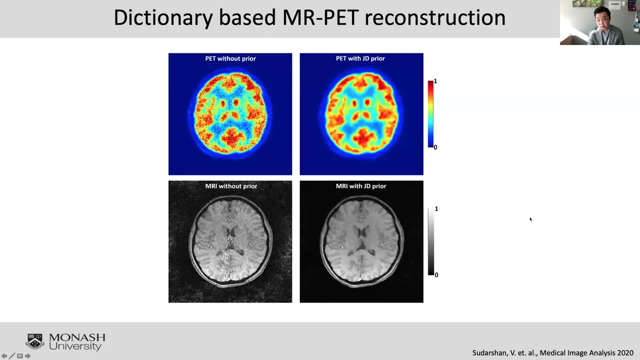 So the dictionary as a function for MRI and the PET. And here's the result. The impact of this dictionary-based reconduction can be clearly seen in PET in terms of reducing the noise amplification, because the MRI is much higher spatial resolution and the signal noise 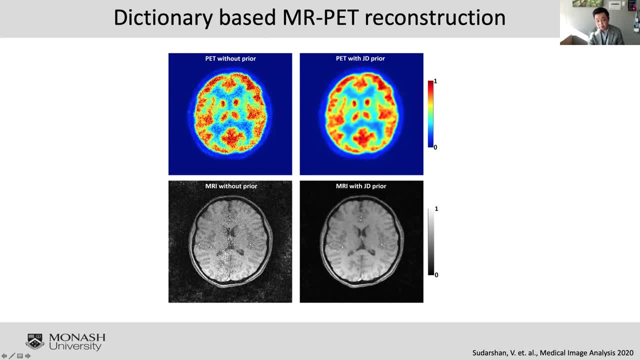 But if we accelerate MRI we have artifacts right. We know the aliasing artifacts and the parallel imaging artifacts will occur if we speed up MRI acquisition. So if we do a conventional image reconduction without the dictionary, it shows a noise playthrough. 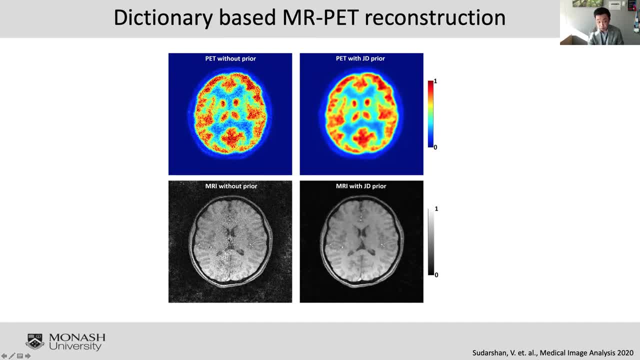 especially in the center, where the condition number of your inverse system- we're talking about before H- is very poor. the noise would be amplified significantly in those locations. We eve used the broad dictionary. This can be substantially improved and the information is actually coming from PET. 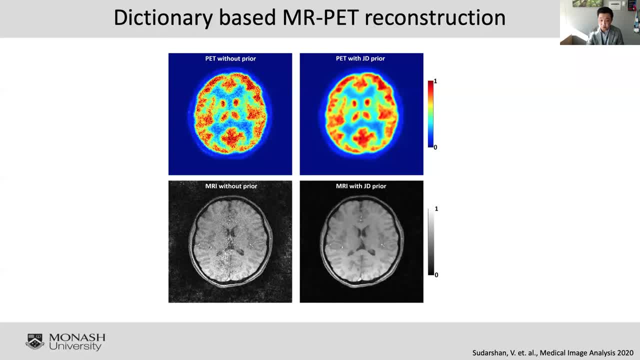 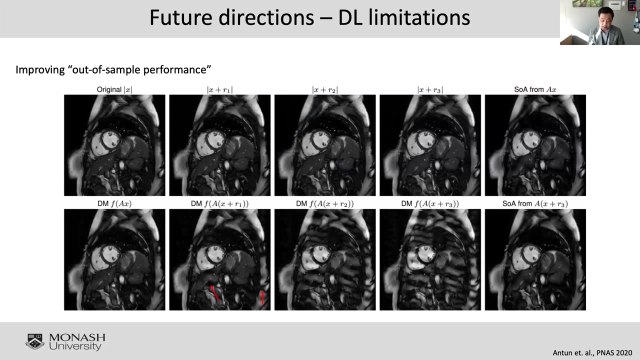 So in a way, MRI is helping PET's reconduction, but also PET is helping MRI reconduct right during this process, the simultaneous reconstruction process. So now these are the recent update around machine learning for biomedical image reconstruction. I want to briefly discuss the future directions of using MRI, using deep learning for MRI reconstruction. 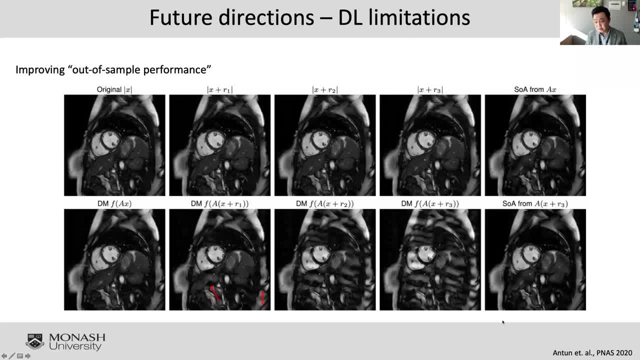 So this is a work from Anton recently published in NPS and they demonstrate there's instability issue with deep models compared with conventional models. So they have done an interesting experiment where they perturb, So adding a small perturbation in the input image. So as you can see here in top row where these are the input, 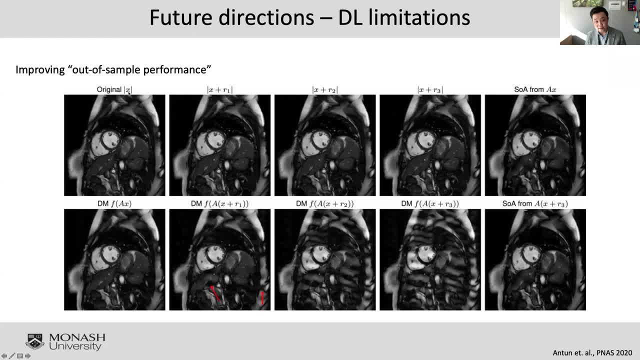 image. So, as you can see here in top row, where these are the input images images, so original images called original X and then with different levels of R's included. so R means small perturbation. you can't really visually see any differences in the images. 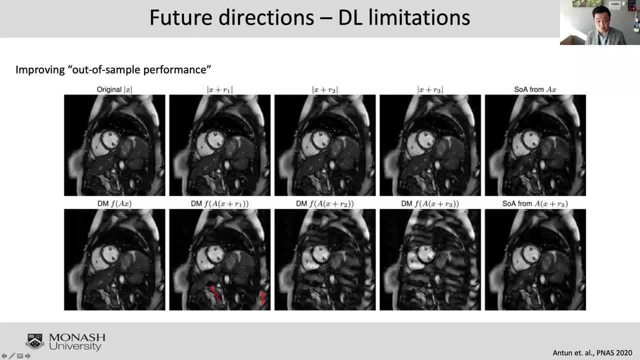 because they are very small, but once you fit into the reconduction network. so the original X seems to be reconducting really well and with conventional technique the last column reconducts really well, but with deep learning it may become unstable. you 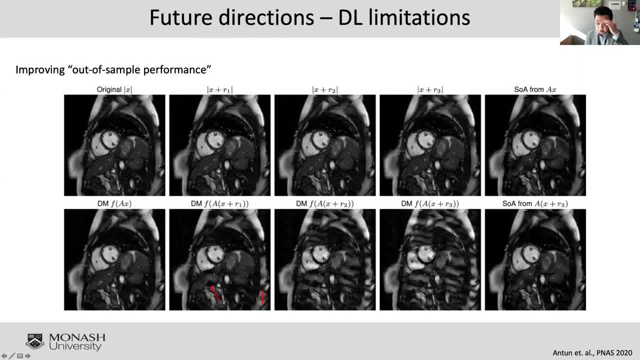 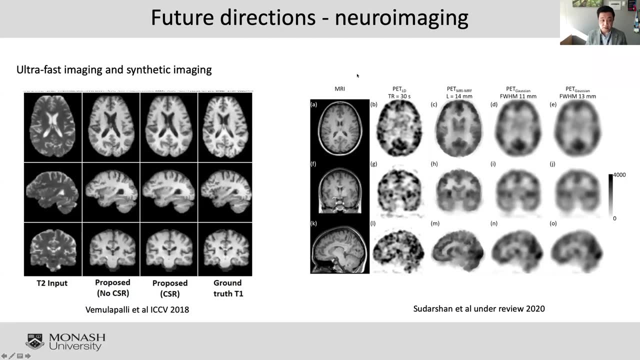 see the artifacts showing up in the image. so this is one of the areas in the community we want to address. it's a stability issue. the other way out-of-sample performance need to be addressed. Another interesting direction for neural imaging in particular is ultrafast imaging and the 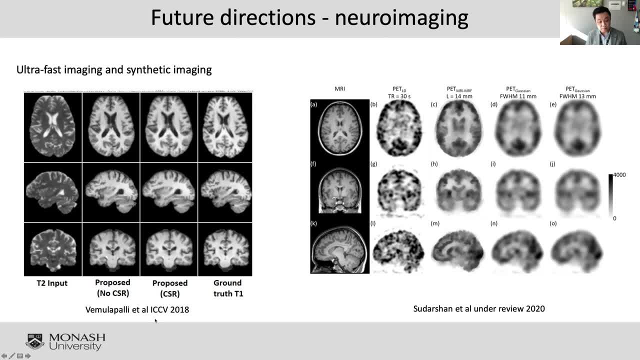 synthetic imaging. This is interesting work. This was published in ICCV in 2018, where they have they used T2 to reconduct T1, to synthesize T1 image without any acquisition of T1 contrast at all. so they demonstrated. 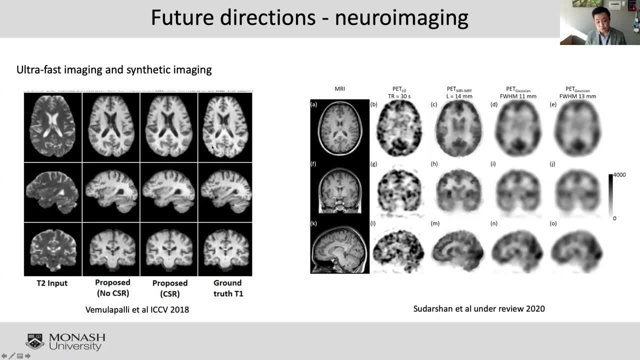 the reconduction similar to T1 as you compare with the ground truth. This type of work still needs a lot of work. Yeah, It's not necessarily quantitative validation, but it's a good starting point. It's a very interesting starting point. 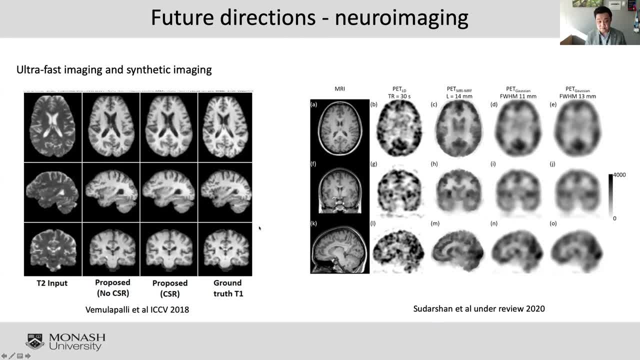 That will help with the further speed-up of MRI acquisition and reconduction. So we also made some effort in this space. so we tried to improve the PET reconduction, For example. in this case we have a simultaneous MRI and PET. The PET is 30 seconds binning, which means the signal noise is very, very low. 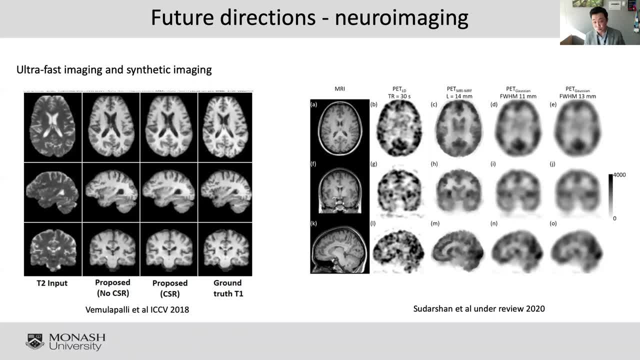 Conventional PET is 20 to 40 minutes. In this case we only do 30 seconds. So, as you can see, the image is really low resolution, high noise. But with MRI we can improve the image quality substantially. so joint reconduction based. 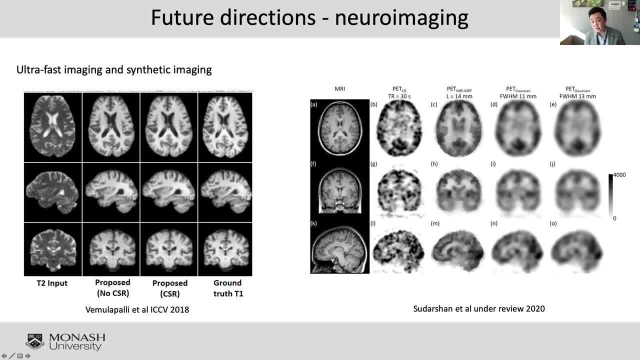 on machine learning, deep learning, And improve the image quality, PET image quality in particular here substantially, even with the 30-second reconduction. You can see from this middle column the third column here, which is joint reconduction And if you compare with conventional smoothing with very high kernel, the image quality still 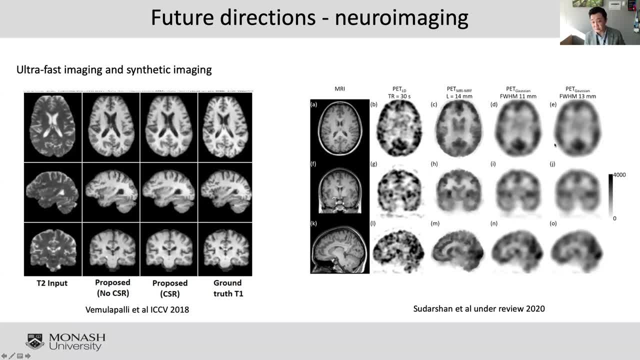 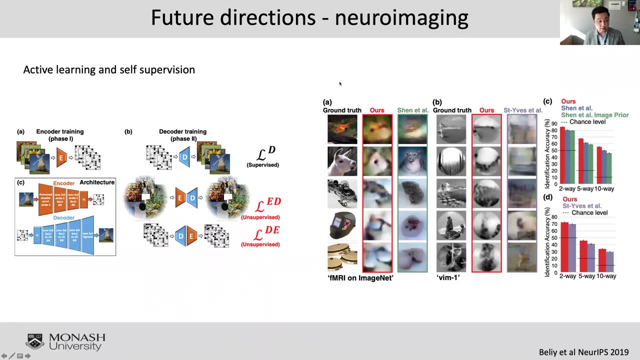 improves compared with in terms of the accuracy, spatial localization of structures is much more better. It's much better defined with this joint reconduction technique. So another area for neural imaging is the active learning or self-supervision. It's very interesting. 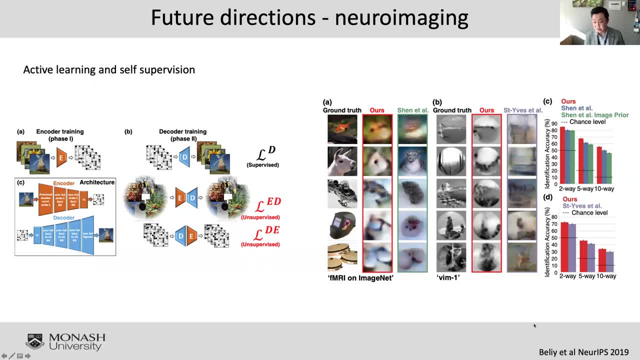 So Bailey, in 2019, published this work in NeurIPS. So basically, they tried to map a natural image scene with fMRI recordings. Conventionally, people do a supervised, a completely supervised way, which means you have a pair of 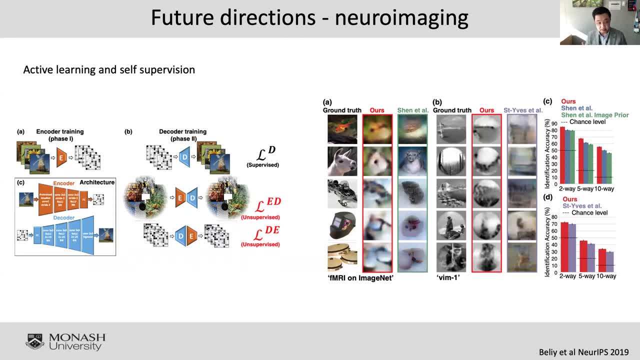 Natural stimulation stimuli, and then the fMRI recording and then you map the relationship between the two. However, the limitation is we don't have such recording and it's not very generalizable. So they developed this two-stages approach. 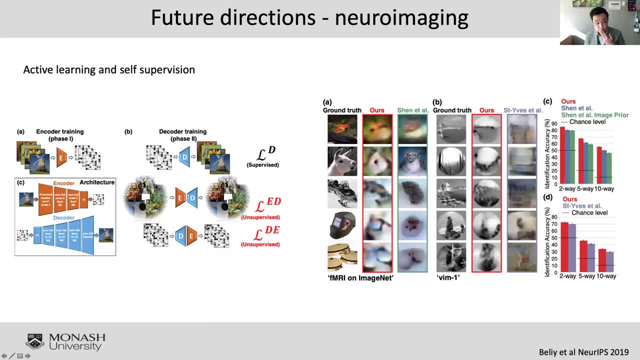 We do first the supervised way and then we do unsupervised learning. So natural image to natural image, fMRI to fMRI. So the importance of this So this is that we don't need training anymore. So let's say, you have a fMRI experiment following their imaging paradigm. 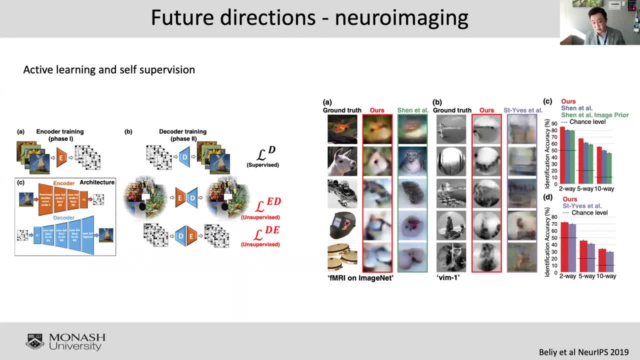 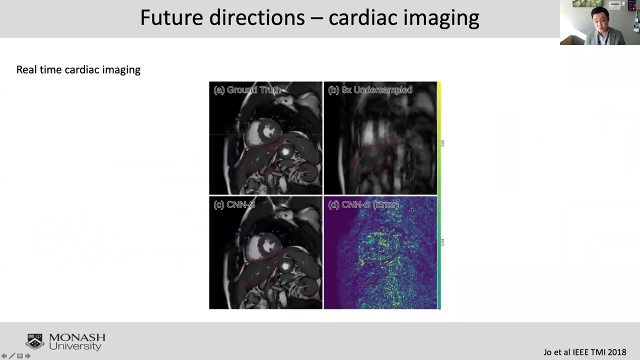 You can potentially recognize the images, reconstructed the images So they compare their approach to data sets and demonstrates the more accuracy compared with the conventional literature technique. Okay, Okay. So the last area I want to highlight is the potential for deep learning in cardiac imaging. 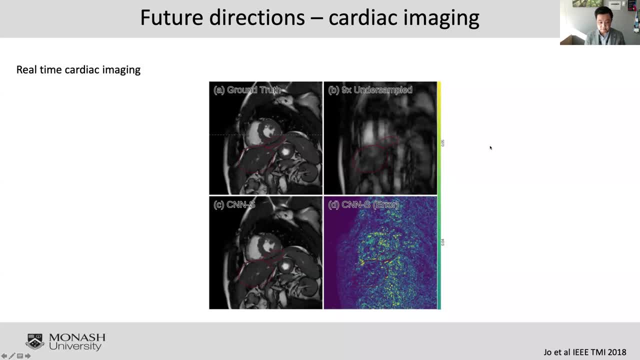 So cardiac imaging, deep learning, sort of natural fit. So cardiac imaging requires, especially for real-time imaging. it requires much faster data acquisition where the conventional technique or having problems reconstructing. as you can see, the image quality is a lot poor compared to the conventional technique. Okay. So then we have some of the high-tech lab and the low-tech lab. So we're performing modest, low-tech, very high-tech programs. So we're actually doing some very good work with those experiments that we do And we're doing a lot of work with the patient- hypersensitivity, the patient-抱able imaging. 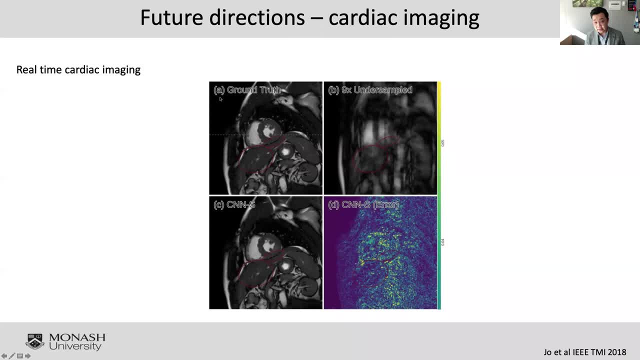 assessment. So we're working on that process, so we're working on some of the best care that we have for that up to this point. Okay, So how does this compare to the gated image showing in Panel A? And if you use a deep learning approach, a convolutional neural net, you can reconstruct. 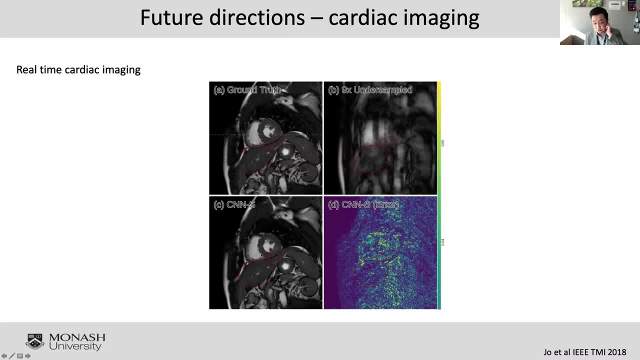 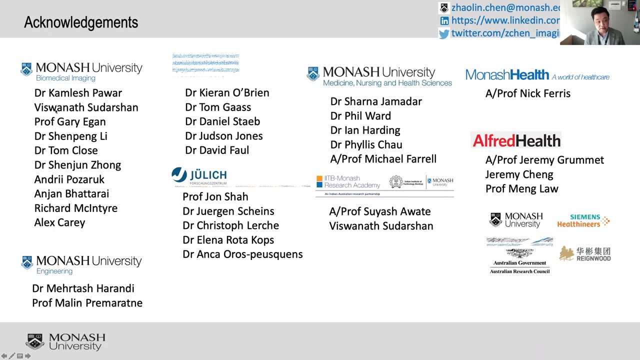 the image as nine times faster, but the image quality is very similar to the gated image, So there's definitely a greater potential in this area. So that's all for my presentation, And I would like to acknowledge our panelists, our ChemNash and Wismana, for their work, and our collaborators from Siemens. 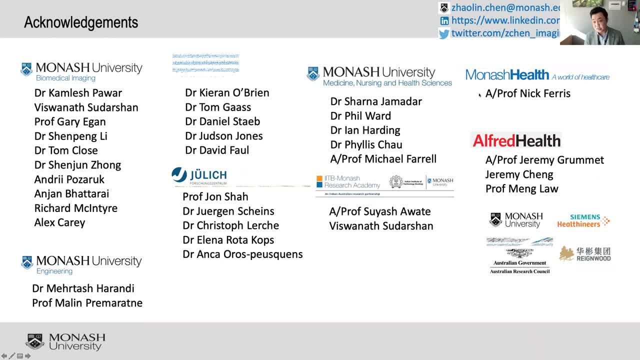 and ULIC, and our internal collaborators within Monash and Monash Health and Alfred and our funding agencies, and also, if you have a question, you can contact me. my contact details are here as well. okay, so that's all my presentation. thank you for a great presentation, Xiaolin. we have one question on the 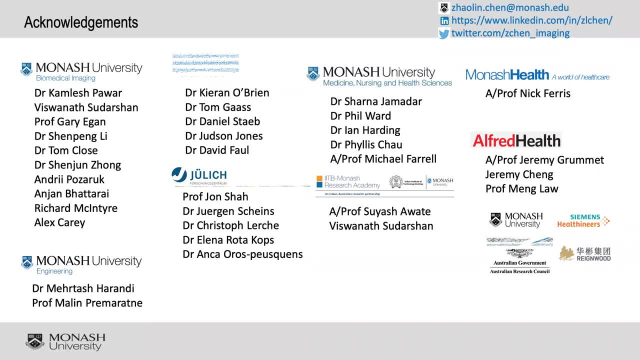 Q&A panel. hopefully people are busy typing others, but I'll just ask you the question from Stefan Bollmann. it's a thank you for a great talk regarding synthesis of contrasts. I often struggle to see the validity of synthesizing contrasts, for example t1 from t2. the information is simply not in the 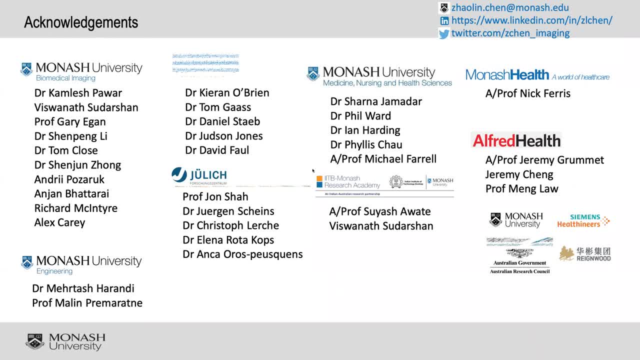 measure data and he's asking you what you think the benefit of this could be. that's very good question, Stefan. I think you point out you know correctly, if the information is not captured, what are the value of doing that, whether it's truly possible. I think the first step could be we reduce the acquisition of the t1. 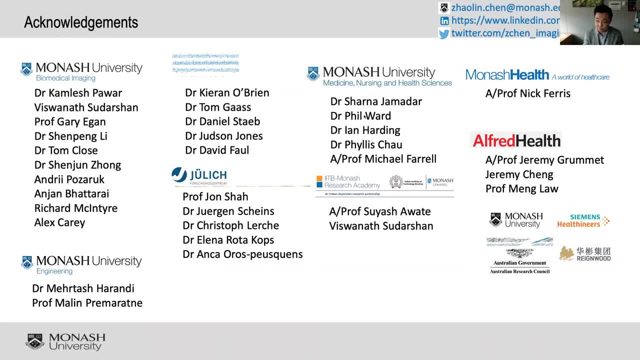 poison. in their case we do a, you know, a very fast t1 acquisition is really minimal amount of data acquired and the lavish, the contrast from T2 to recontract the T1. so this is the area and still needs a lot of validation and continuous experiment work. 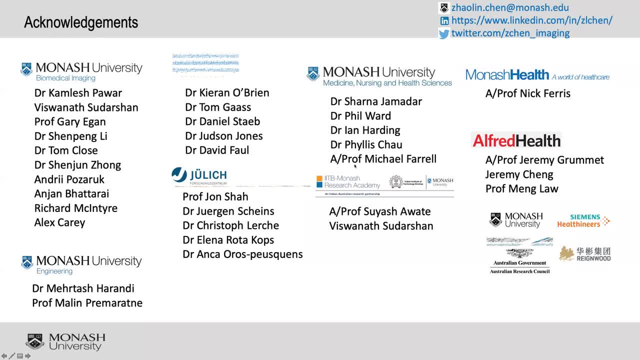 thanks, Sjerling. I have another question from Timmy. can you talk more about the perturbation effect? what was the perturbation and how does it affect stability? right so the perturbation. the perturbation and how does it affect stability? right so the perturbation. 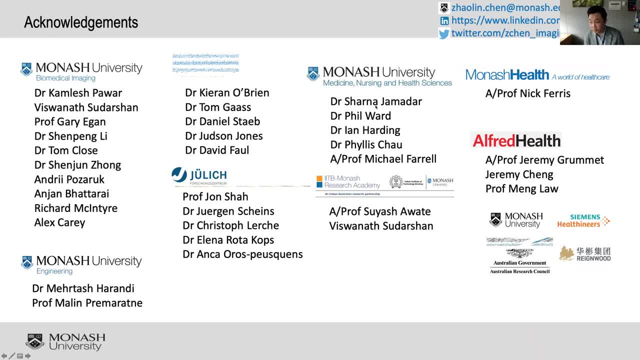 experiment. what they have done was they try to search, let's say the. the network parameter has been identified, so after that they try to search whether there exists. a small perturbation can change the input and output difference, so which means a small change in the input will cause a large. 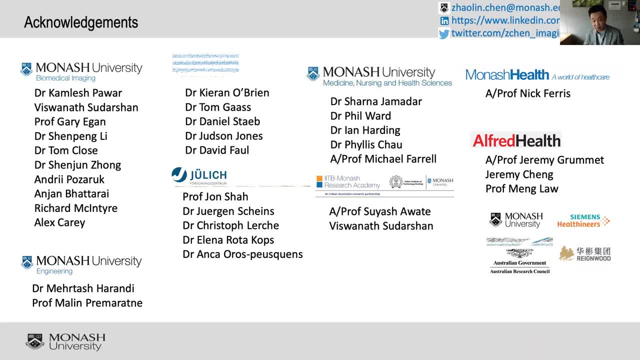 effect in the in the output. so they actually design optimization problem in such way and to to test the stability of the network. thanks, generally, if you have any follow-up questions, particularly if you've asked a question, just type them in the Q&A and I can read them out as well. I guess, like I have a question. I. 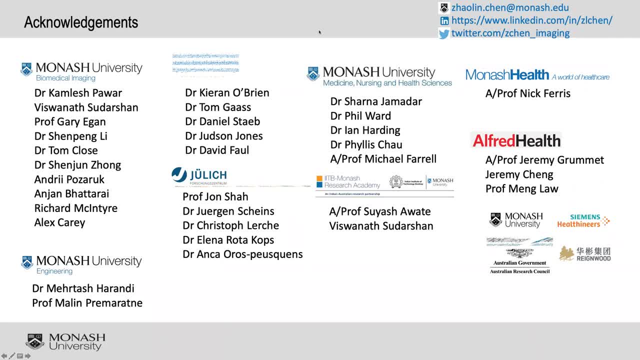 can't seem to type in being a panelist, so I'll just ask it verbally. I think a lot gel in. I think that was a great overview, really beautiful work, and it's amazing to see how quickly, I guess, the quality of this imaging is improving with with with deep learning and machine learning approaches. I guess my question 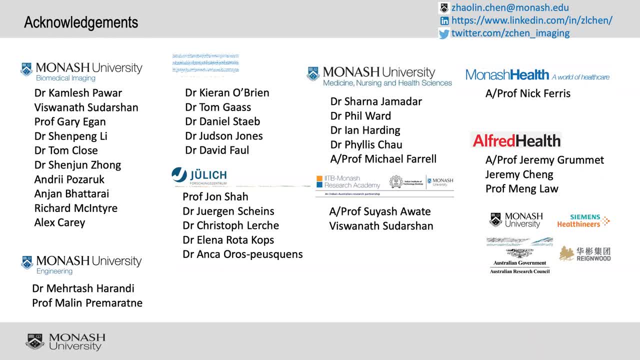 to you. I've got two questions really. one is around this: out of out of sample performance and the stability or instabilities associated with that, like that can really create major problems for the application of deep learning reconstructions, and I just wondered if you could reflect a little bit more on 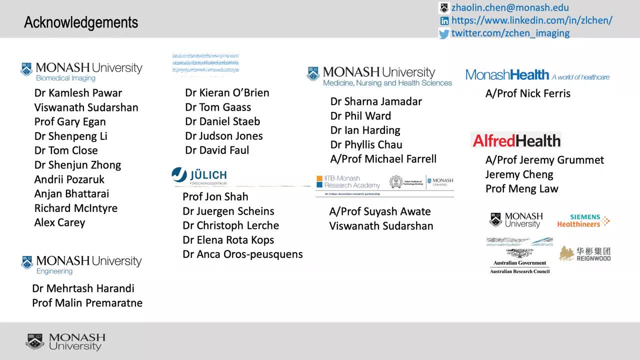 whether you think that is ultimately going to be sort of addressable or do you think that there's going to be some major pitfalls with having instabilities because of out of sample, out of the training samples. and the second part of the question is around just how big the datasets need to be to do good training. 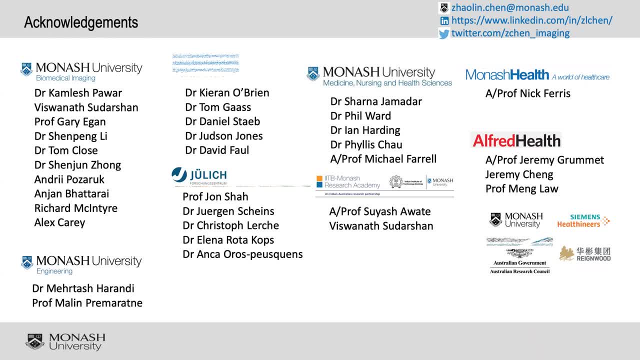 or at least the area I'm working in, is out of the training samples, and the second part of the question is around just how big the data sets need to be to do good training, or at least the in those applications you showed that involve having training data sets. 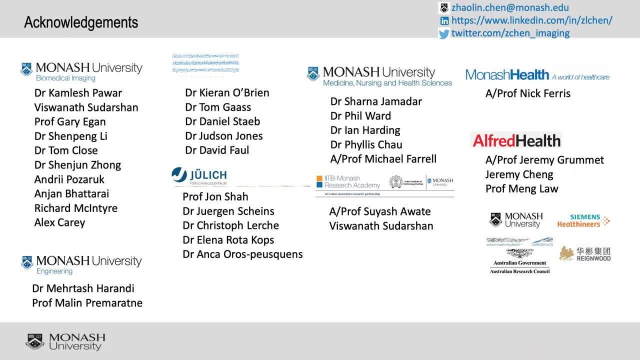 Are we talking sort of hundreds or thousands, or how many data sets do we need to get really robust deep learning reconstruction models? That's a very good question, Gary. I think you pushed the boundary of the deep learning research here. So I guess to answer the first question, 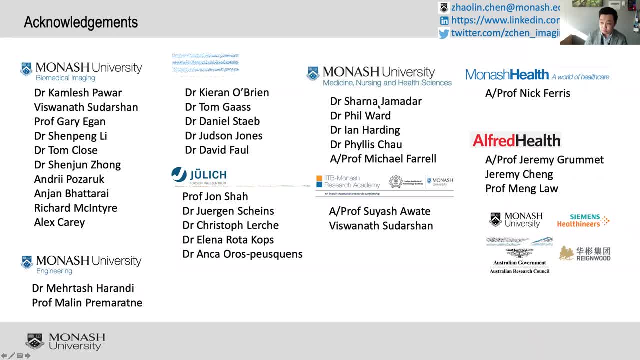 whether stability will be a fundamental issue for deep learning or not. I think the community- beyond imaging, I mean the deep learning community- is trying to address two issues fundamentally. One is: can we make it generalizable and can we make a deep learning rather than black box? 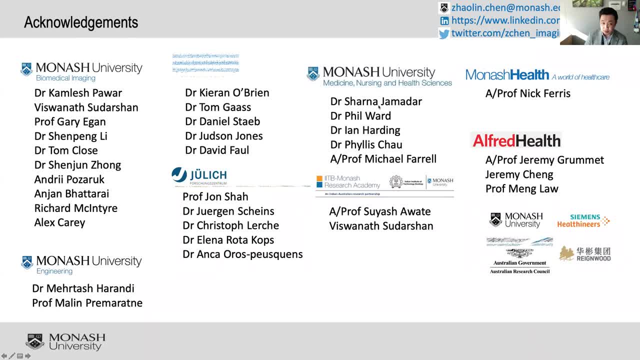 to make it explainable. I think along those lines, a lot of the model parameters, we get a clear and clear understanding. So that's one aspect we can certainly will certainly help the out-of-sample performance problem. Another aspect of this, so, and also our work in terms of camera careers, work. 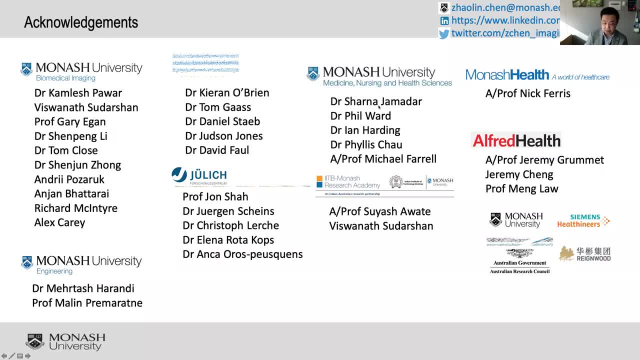 we try to use physical knowledge to augment the deep learning models where we can generate- maybe this is also linked to the second question, Gary- So we can generate a lot of new data which will enrich the model information using the physical knowledge. So we can, for example, the motion. 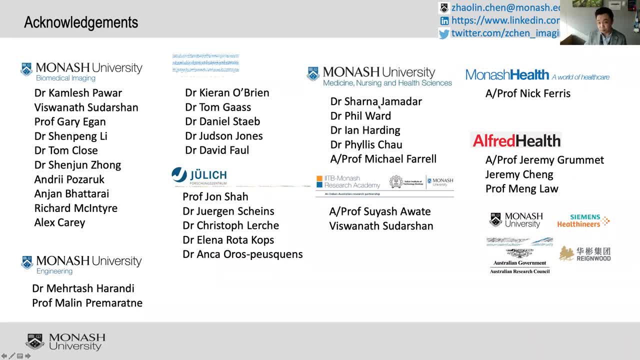 we can simulate the motion artifacts. I think people also develop different techniques for, for example, QSM. You can simulate. that's probably Stefan's work as well in the to simulate QSM samples to train a deep learning model in that way. 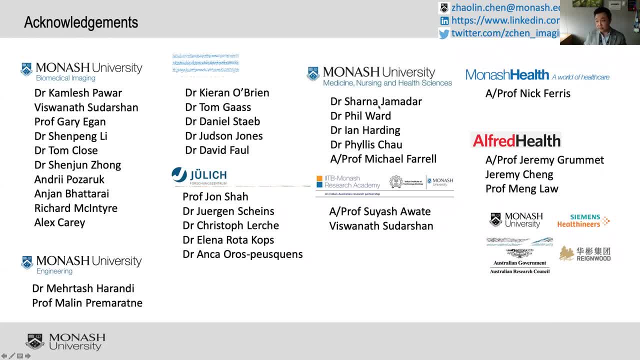 So that I think they acquire data plus the simulated data can create- you know a, you know a deep learning model in that way, So that I think they acquire data plus the simulated data can create a deep learning model in that way. 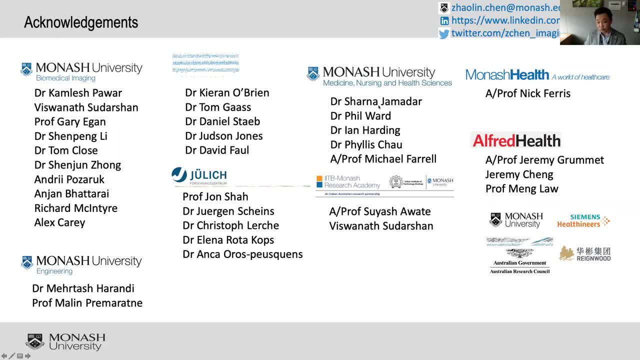 So that I think they acquire data plus the simulated data can create a deep learning model in that way, So that I think they acquire data plus the simulated data and have a unique opportunity for solving a lot of these issues. But what is correct is the deep learning. 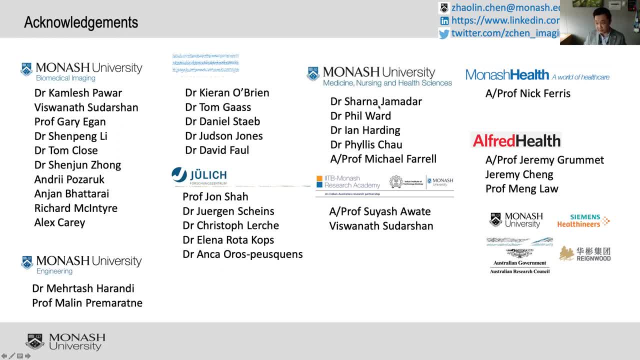 has millions of parameters compared to conventional physics based modeling, which has only 10, 20 parameters. So we can think about millions of parameters against 20 parameters. a million parameters, you know substantially larger amounts of data to train. Yeah, exponentially larger. 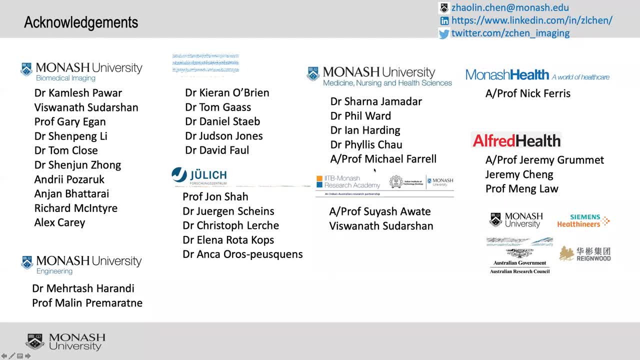 Right, thanks. Matthew has another question similar to the one I was going to ask: is the end-to-end deep learning reconstruction actually justifiable in terms of processing time? That's another good question, Matthew. So the automatic work and also our end-to-end image reconstruction work, the training from 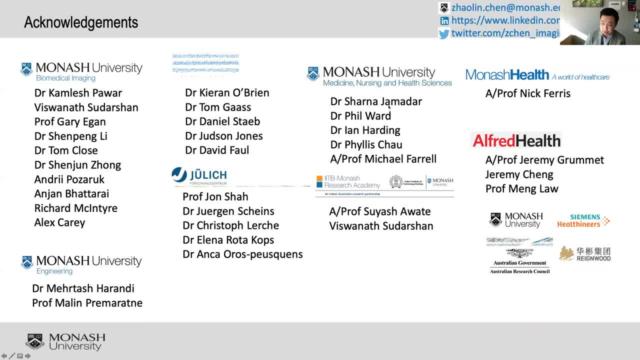 end-to-end definitely a lot time-consuming, especially the automatic work. They have a fully connected layer to map the Fourier transform, So that's also one of the limitation of their work. they can only apply to small datasets. you can't reconstruct large images. 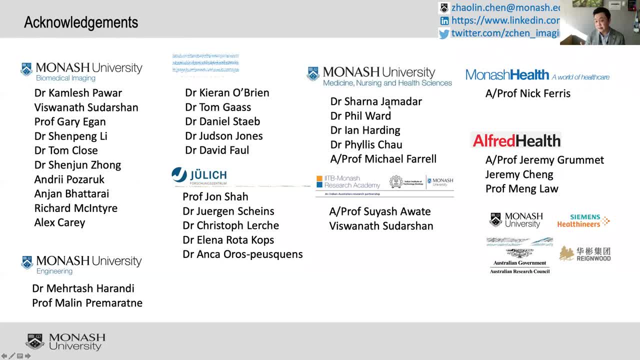 But once you train the model- let's say you take a few hours a day- train the model. once a million parameters been estimated, the inference of that model is actually in few seconds. It's not that bad at all. Okay, thank you. 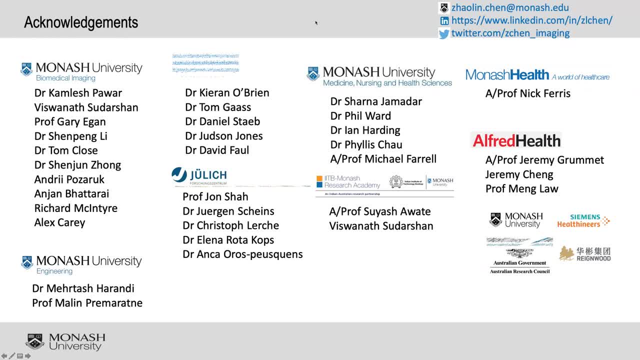 There's no more questions in the Q&A if anyone wants to quickly type one in. I was interested in the dictionary-based PET-MR reconstruction. I assume that would be tracer-specific. Is there any chance to train those to be usable across multiple tracers? 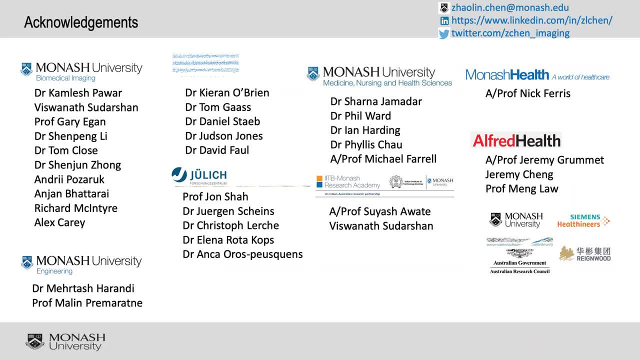 to guide the MR reconstruction. Yeah, that's a very good point. So it will be tracer-dependent. The mutual information between different PET tracers, I would say, is the instrumentation aspect. So the detector modeling, the bio-distribution of the tracer will be different. 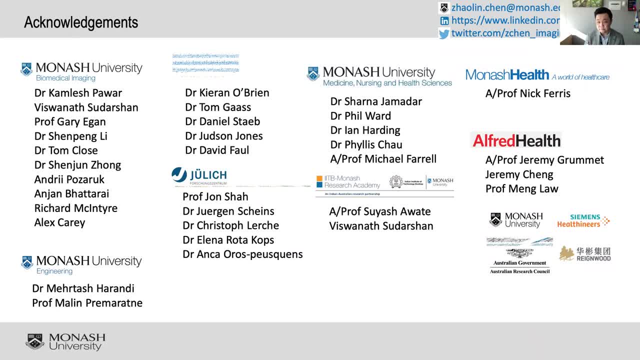 So there is opportunity to model the physics, underlying physics, instrumentation aspect as using dictionary, But on top of that it need to be a tracer-dependent model to adapt for each tracer. I think that's how it should be done. All right, Just Ted. one last comment. 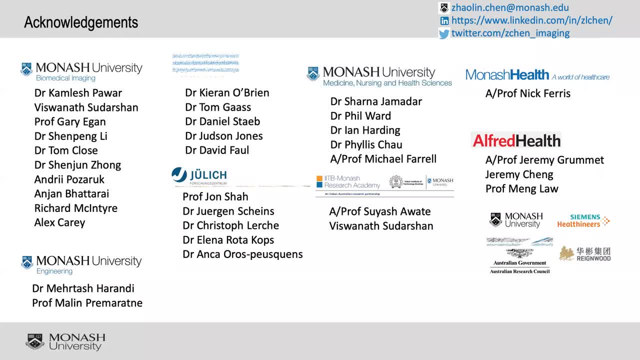 Xiaolin, whether or not you had thought about you know, whether or not you had thought about you know, whether or not you had thought about looking at total body PET image data, which can, of course, with the incredible sensitivity of those total body scanners. 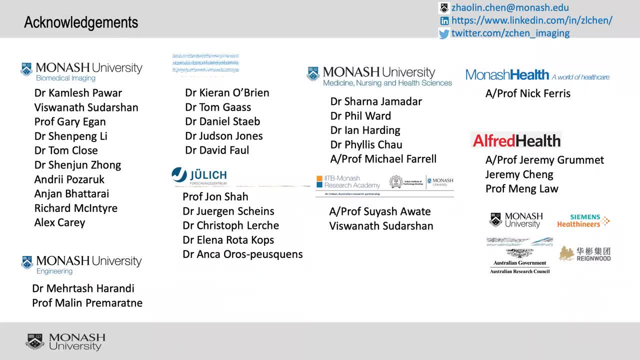 can provide data with very, very short or sufficient counts and data in a very short time interval. Have you considered that for deep learning applications And, if so, how fast do you think you can get a whole body, total body, PET image? Yeah, 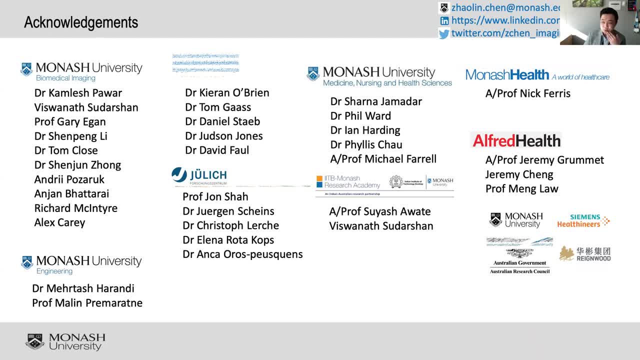 Yeah, we haven't. I haven't really think about that, but that's good point. I guess if we can reduce the PET dose to a minimum level, let's say the speed, then the bad shuffling speed it will be the limitation. 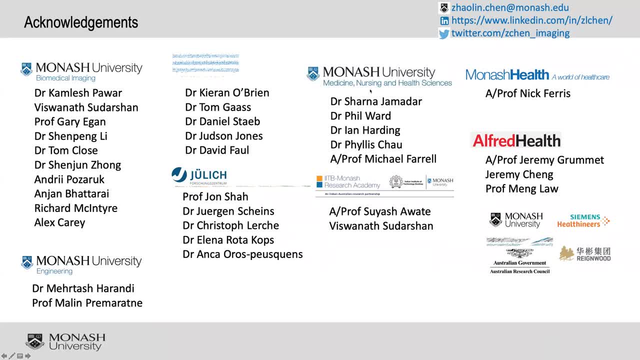 Great thanks. So I guess Matt is asking another very summative question, which is good. We'll leave it on this one, I think. Are you saying that you can see the end of conventional iterative reconstruction? are you saying that you can see the end of conventional iterative reconstruction?